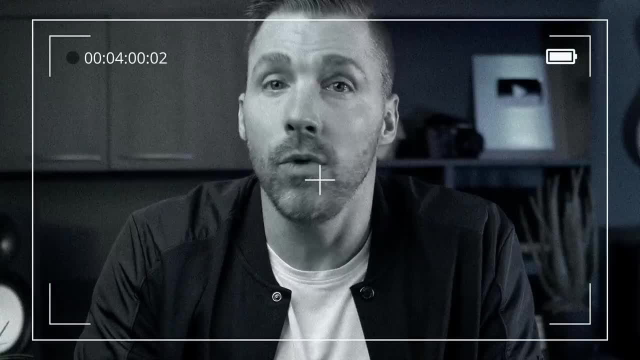 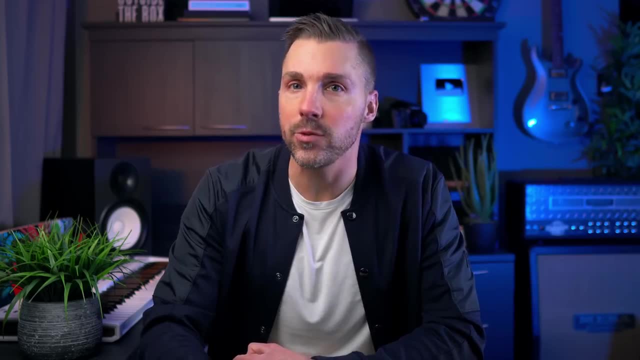 it could be something as simple as you're just going after the wrong segment, or you're going after the right segment, but in the wrong way, using the wrong words and messages and offers. Now, this next part is really important, so I'm going to say it as slowly and clearly as possible. 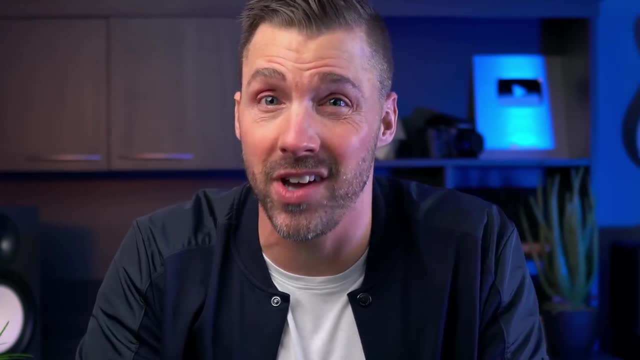 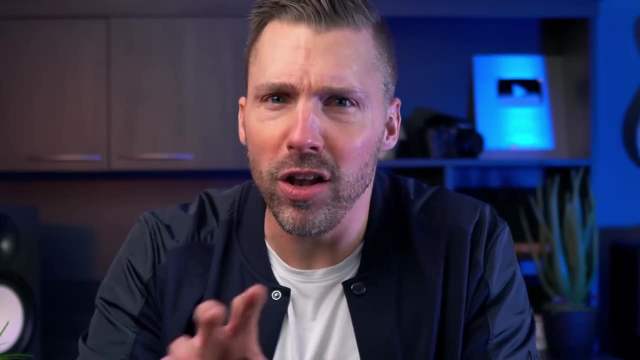 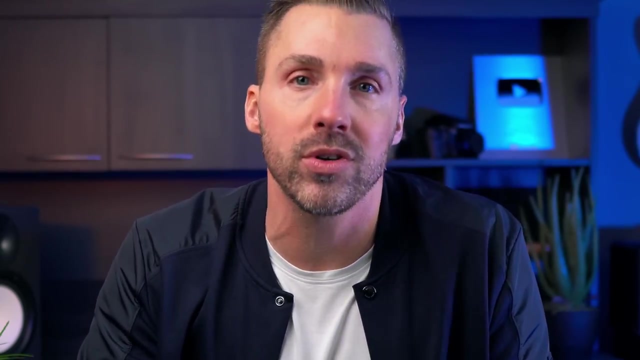 Feel free to pause the video or even rewind and rewatch this a couple times. Matching your message to your target market is the key to success, And getting this right will immediately make all of your marketing ten times, maybe even a hundred times, more effective and more profitable, making attracting new customers and making more. 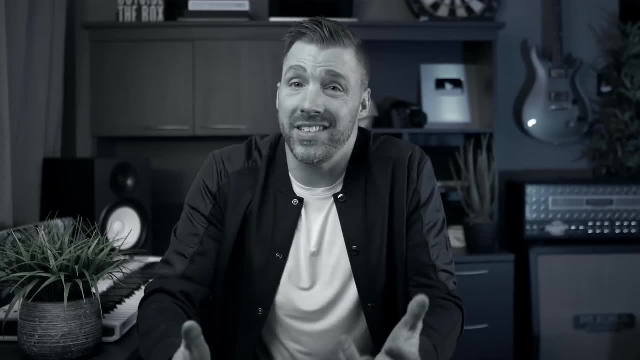 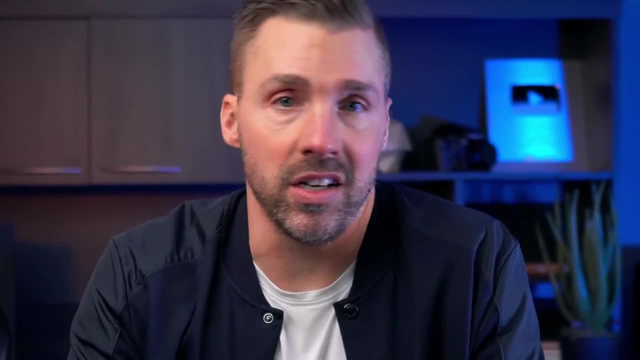 sales easier than ever before, But get this wrong. and well, sadly, this is one of the biggest reasons that most businesses fail, And at best, you're just going to keep going around in circles, feeling stuck and stalled and frustrated and overwhelmed, and I want better for you. 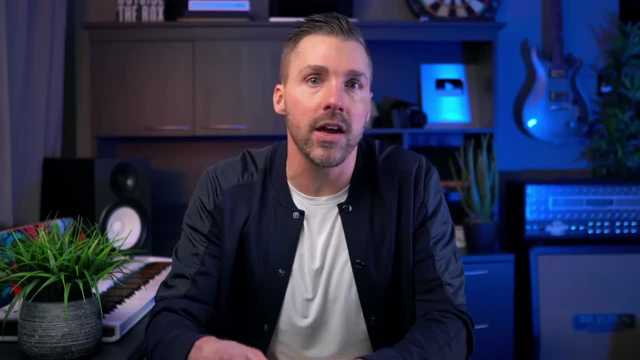 And this is why one of the things that you're going to want to do, and this is why one of the best places to start- any time you're thinking of starting a new business or launching a new offer or introducing a new product or service to the market- is Amazon. 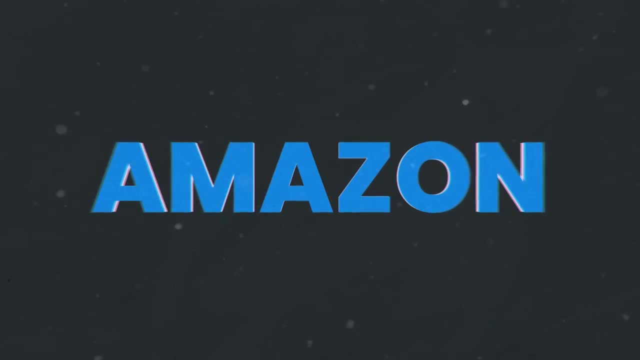 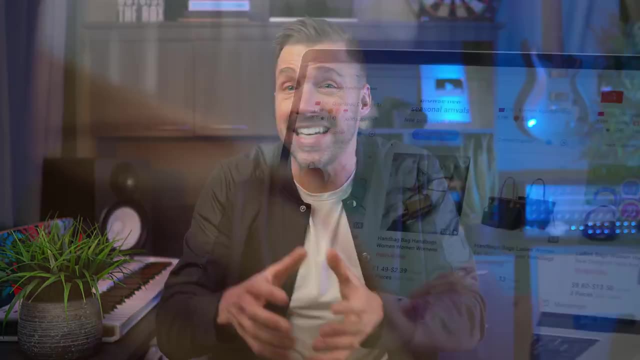 No, not the jungle, the website, and here's why The fastest and easiest place to get ideas, inspiration and do research on both your customers as well as your competitors is Amazon or any other online book retailer will do. This is because books typically take a longer time. 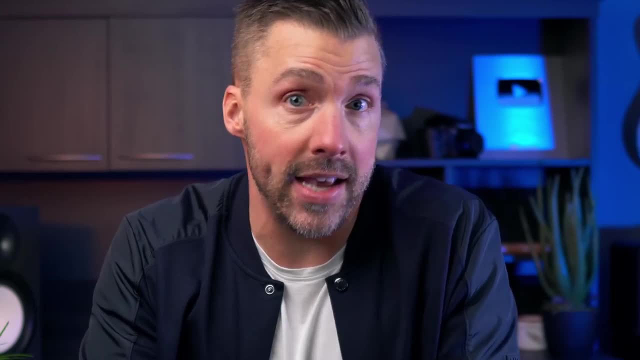 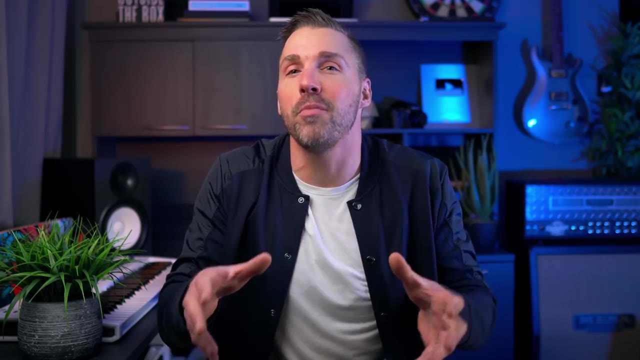 to write and to edit and to publish than most of the other forms of media out there, which means you can be at least a little more confident in the information that's being presented, opposed to, say, basing your entire marketing strategy off a tweet that somebody posted at two o'clock in. 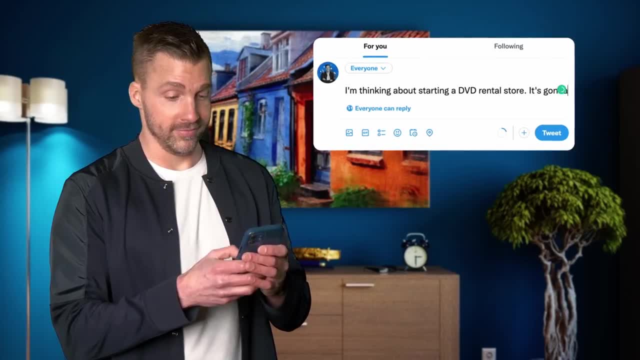 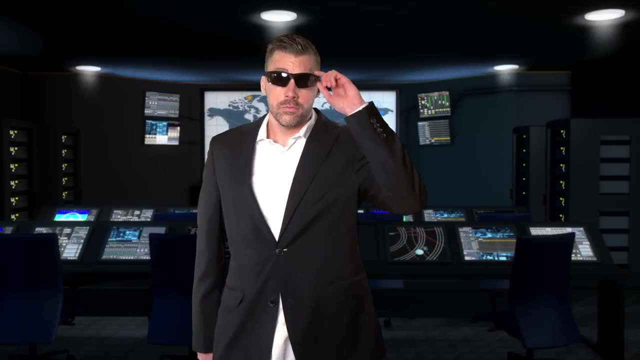 the morning. I'm thinking about starting a DVD rental store. It's going to be huge, bro, But you're not just going to Amazon to browse. you're on a mission, a market research mission, Which, when I say it out loud, makes it sound like the most. 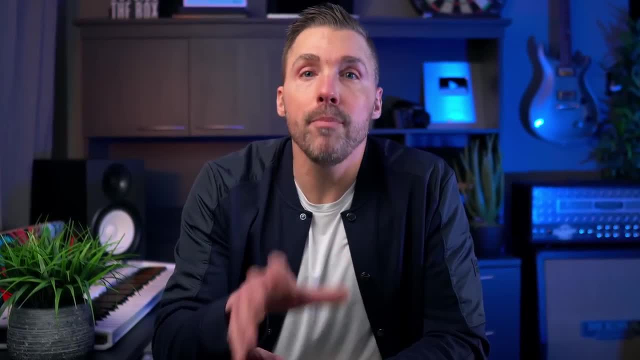 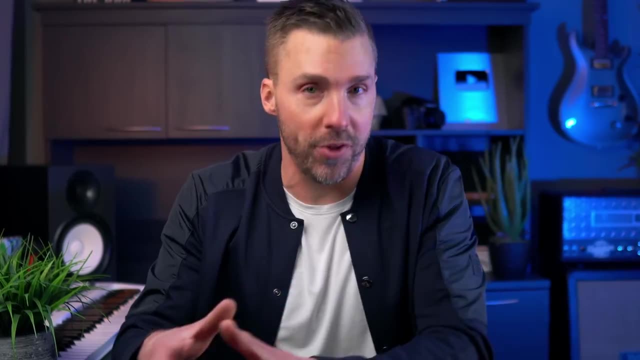 boring mission ever. Anyway, what you want to do here is look up books in your market, your niche or your industry and see what the titles are, what the descriptions say, how many reviews there are and what the reviews say. 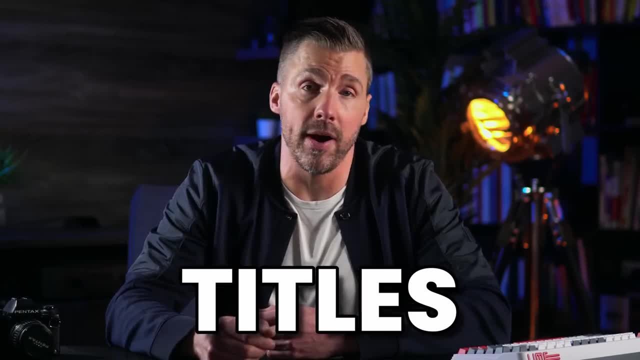 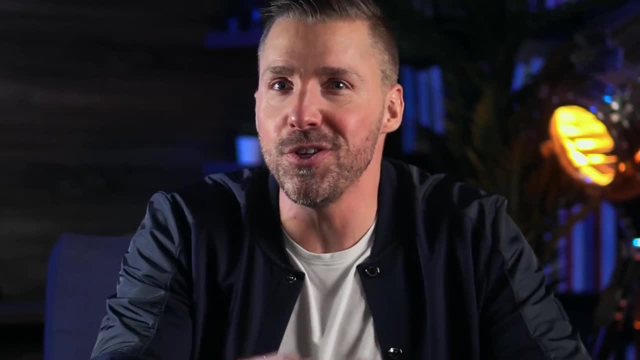 The titles will tell you what topics, angles and hooks people want to read about. The description of the book is basically a mini marketing message and is designed to highlight the benefits of the book, and you can use this to get an idea for how other people are talking about. 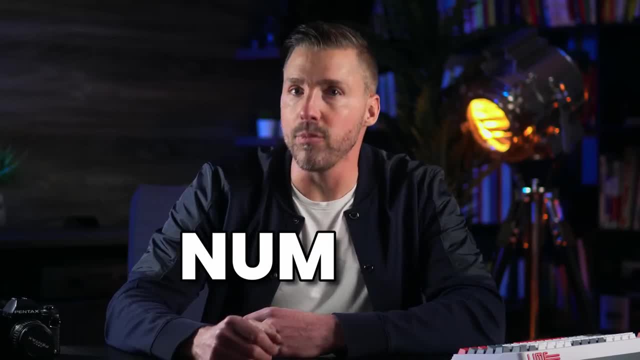 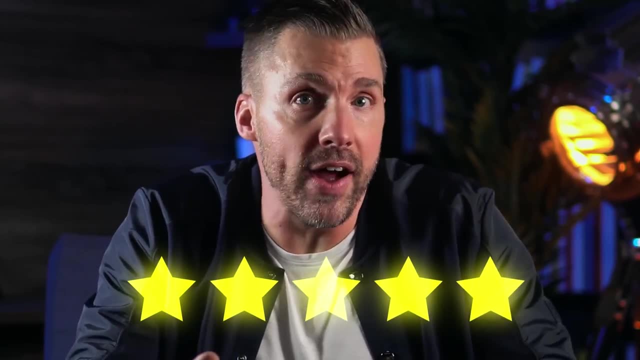 the pains and problems that your customers experience And the number of reviews the book has will show how many people care about the topic enough to actually post a review. Read the five-star reviews to find out what people liked and why, so you can make sure your business offers those same solutions. And read the one and two-star 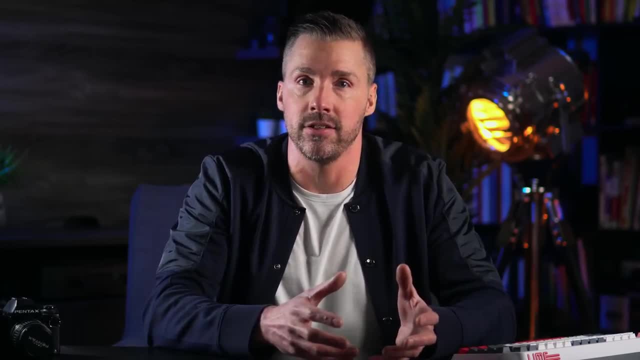 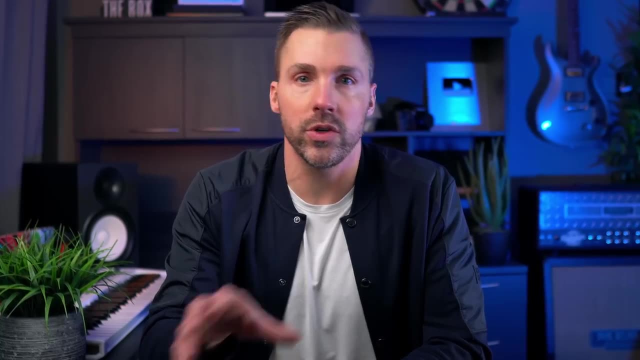 reviews so you can see what the book missed or what people didn't like, so you can choose whether or not to include those things in your marketing. Another thing that you want to do here, not just with Amazon, but with all of the resources and tools and strategies that I'm going to be sharing. 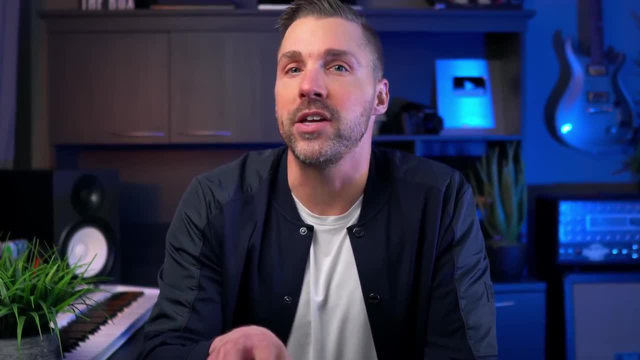 with you throughout the rest of this video is start to use that information to put together an ideal customer avatar. I'm going to be sharing some of those with you in this video, so if you're interested, please do so. Or if you already have an ideal customer avatar, then using the 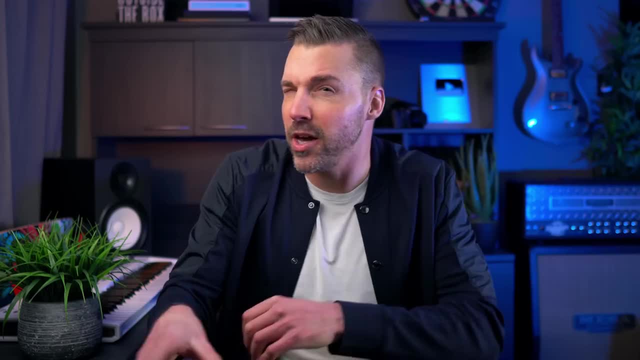 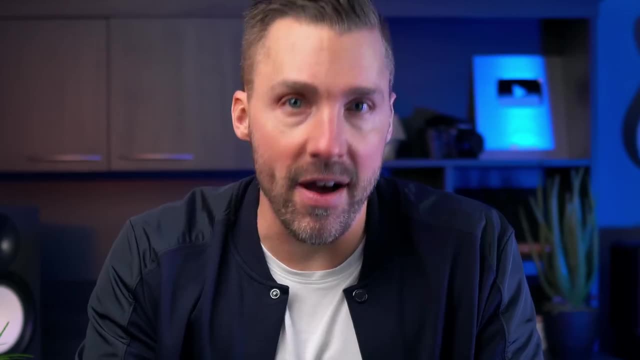 information that you gather and collect and, essentially, research to compare against it in order to make sure that you continue doing the right things for the right people in the right place. Now, if the whole ideal customer avatar thing is completely new to you, don't worry. it sounds way more complicated than it actually is And it's really just a fictional. 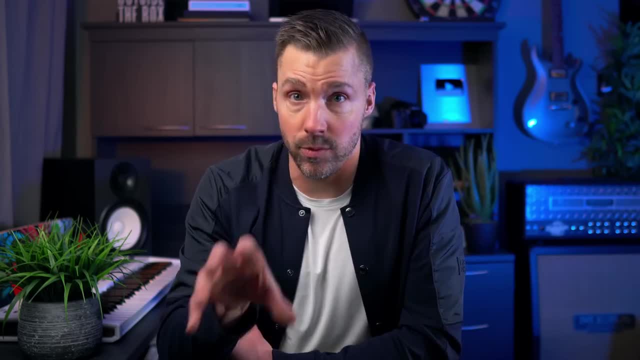 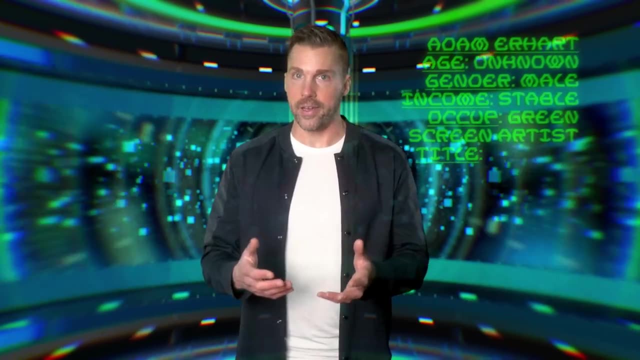 though sometimes real representation of who your best customer is, and it's made up of all of the things that they have in common. These are things like their demographic details, like age, gender, income, occupation and titles. Geographic details like what city state. 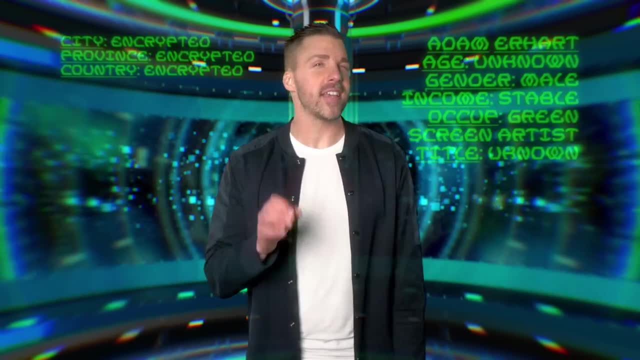 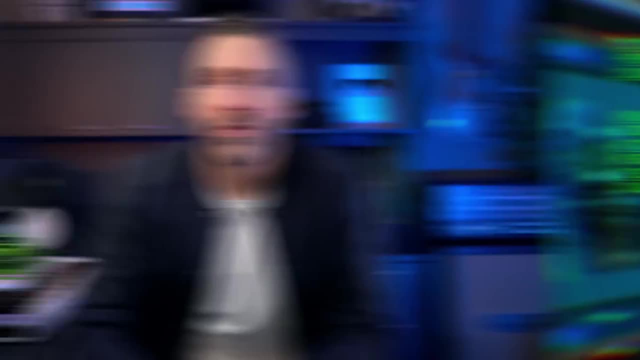 province or country they live in And, most importantly of all, psychographic details like what are their values, their attitudes, their lifestyles, beliefs or any groups or organizations that they're a part of. Another thing you can do is take advantage of and 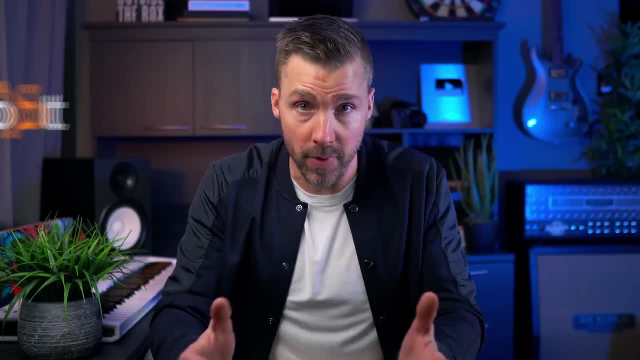 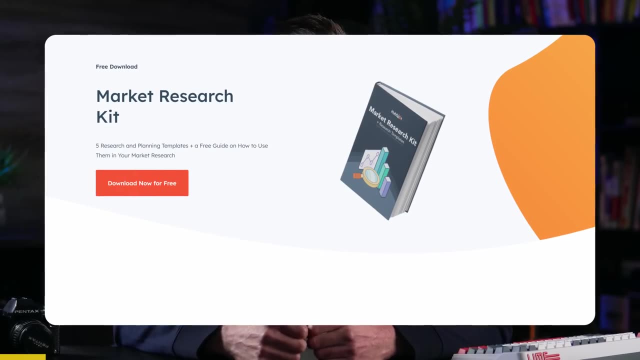 download the free market research kit provided by this video's sponsor, HubSpot. So let me walk you through that now. HubSpot's market research kit is made up of five different research and planning templates and comes with a free guide on how to use them in your 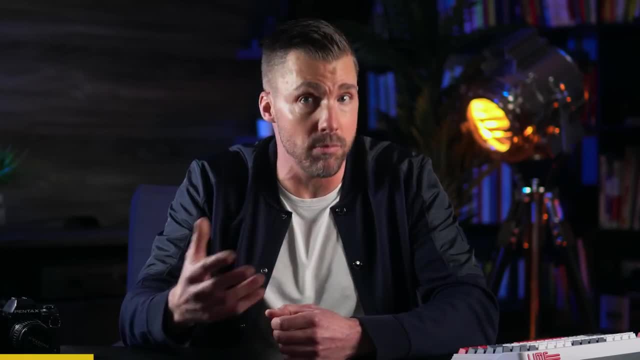 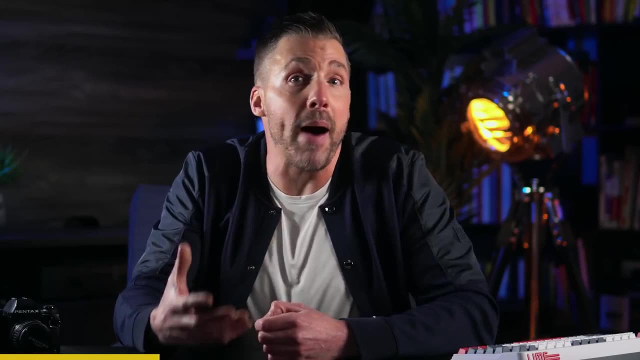 market research and will help you find out important industry and market factors like the market size and trends, the regulations, gaps in the market and market demographics. It can help you build a buyer profile with all the things we just talked about. 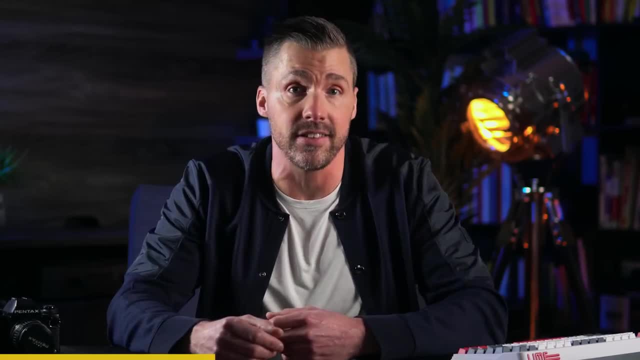 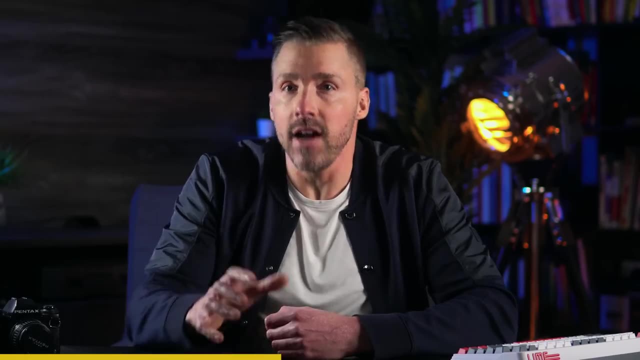 like age, gender, income level, lifestyle trends, needs and attitudes. It'll give you guidelines for competitor research, looking at pricing structures and market share, and marketing and branding, And HubSpot's free market research kit includes an industry analysis. 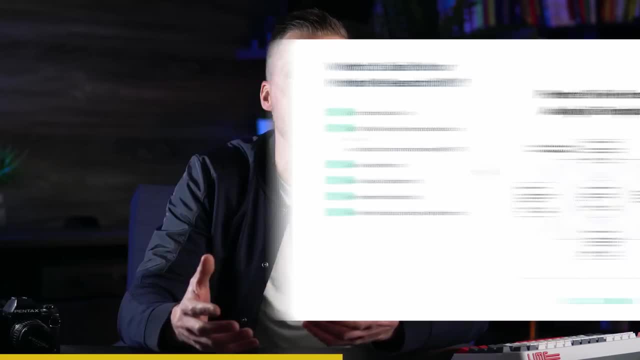 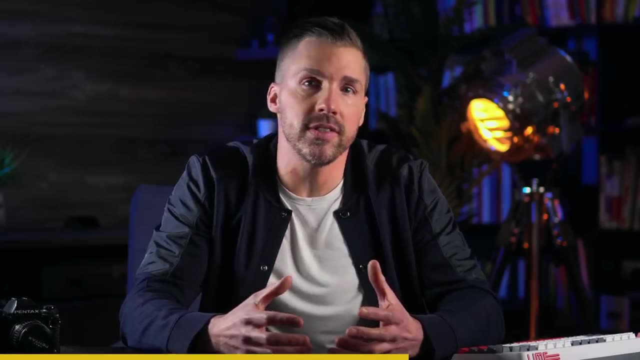 template to kickstart your market research and basically get you up and running as quickly as possible. If you know you need market research but don't know where to start, then start here, as the kit includes an instructional guide, SWOT analysis templates available as Word docs or interactive design, PDFs, a survey template. 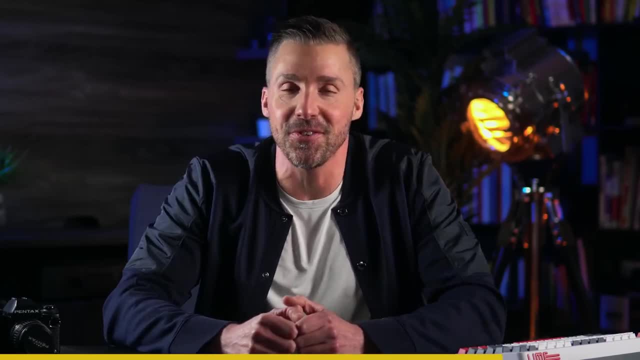 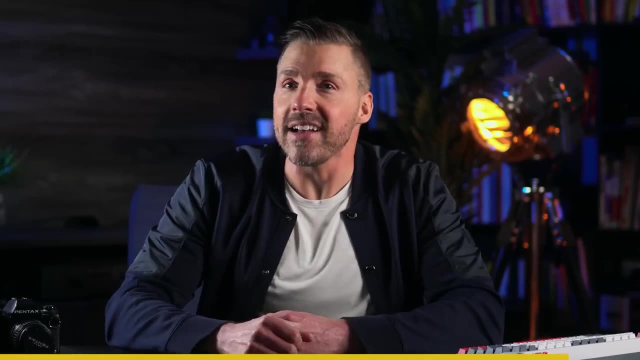 focus group template, presentation template and five forces industry analysis template. So make sure to click the link in the descriptions below right after this video, and download your free market research kit today. Next, let me show you another powerful tool you can use to get access to more data and information than you ever thought possible. 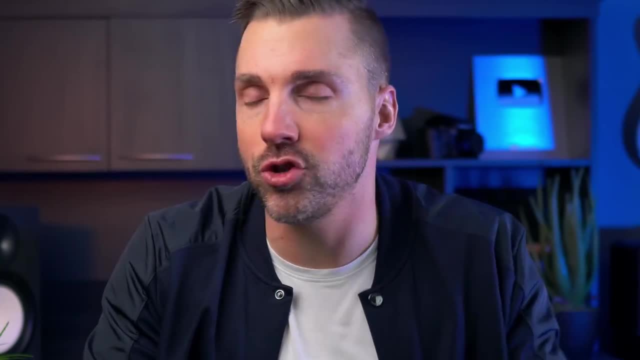 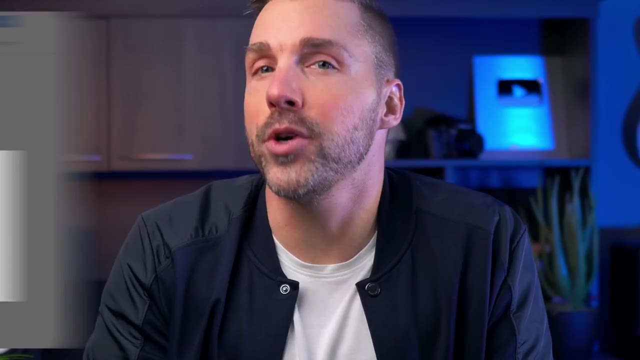 using Think with Google Research. Think with Google Research is a treasure trove of Google-y goodness, But the two things that I want to direct your attention to are number one- find my audience- and number two- Google Trends. So let's start with find my audience first. 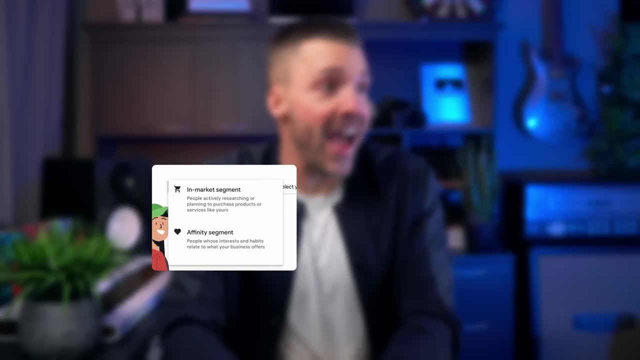 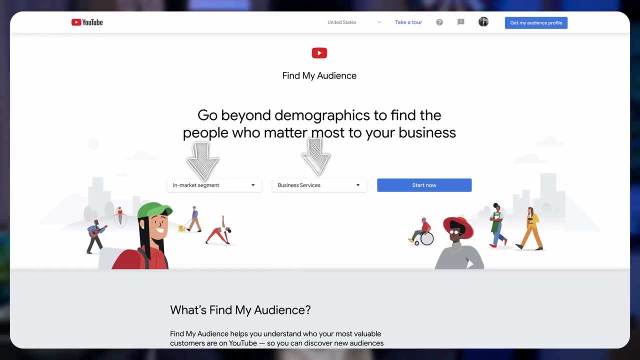 If you've ever run Google Ads before, then it's going to look pretty familiar, as it allows you to look over and dive into different in-market and affinity segments. For example, if I pick in-market and then business services, I can see advertising. 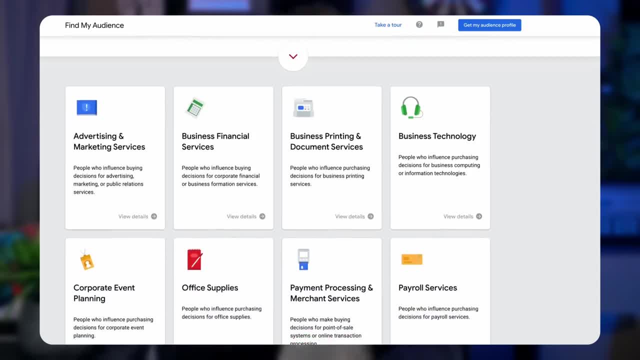 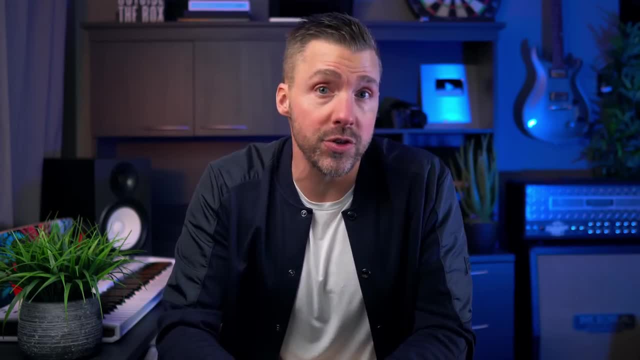 and marketing services, business and financial services, business printing and documents services, business technology and a whole bunch of other business-y related services and topics and products that people are interested in, And I can click on any one of these like say: 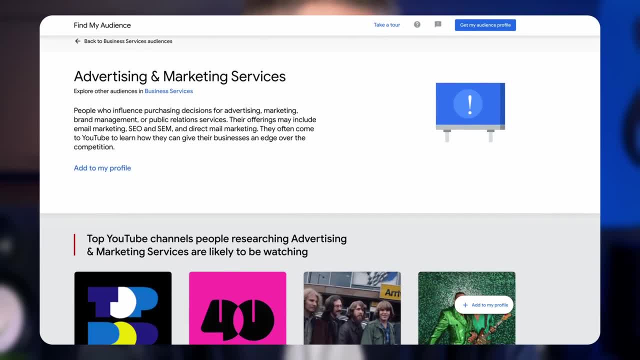 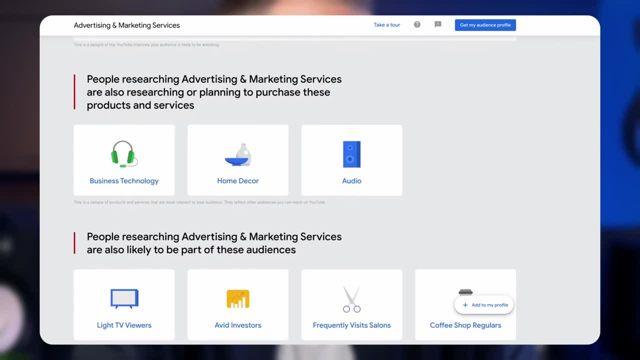 advertising and marketing services and I can learn more about this audience, including what other YouTube channels they watch, what other purchases they make, what other audiences they're likely to be a part of, and other subcategories within advertising and marketing services that I may want to check out as well. It's a powerful little tool, especially when combined with this. 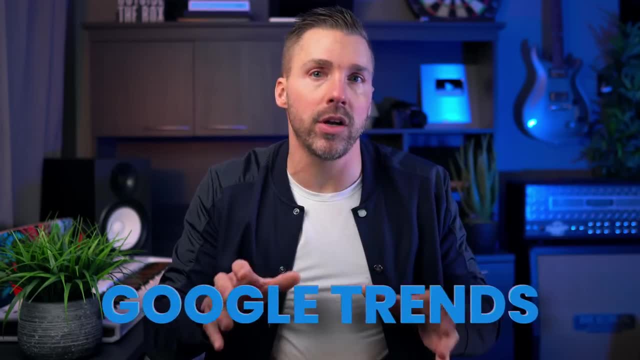 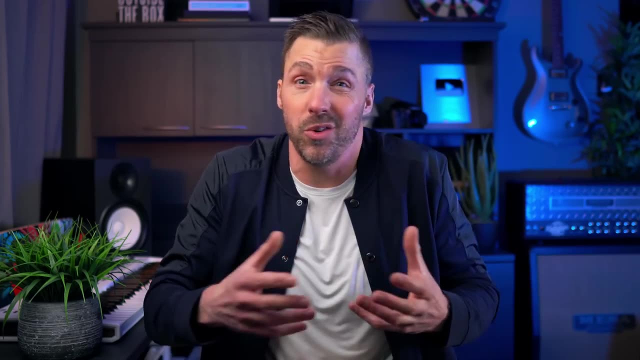 next one, Google Trends. Google Trends is another fantastic market research tool and it's great to give you sort of an overview or high-level 30,000-foot view on a business or topic or industry or essentially anything that may be trending. 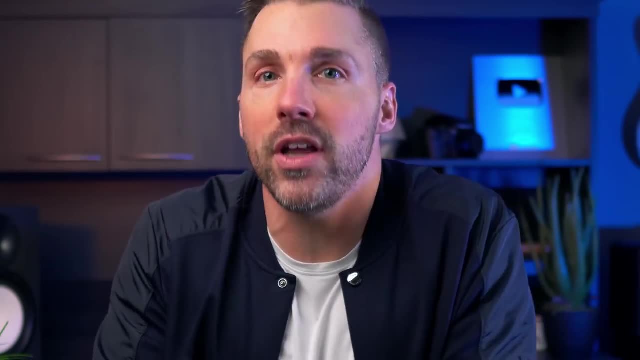 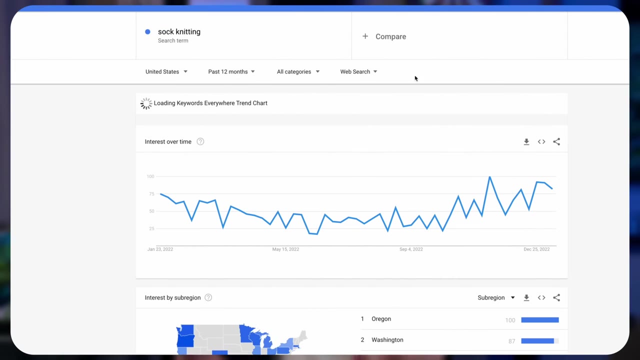 All you have to do is simply enter a search term and it'll tell you the level of interest that this topic has, both now and in the past. For example, let me type in something random like, say, sock knitting, in order to see what's going on in the industry right now. Well, 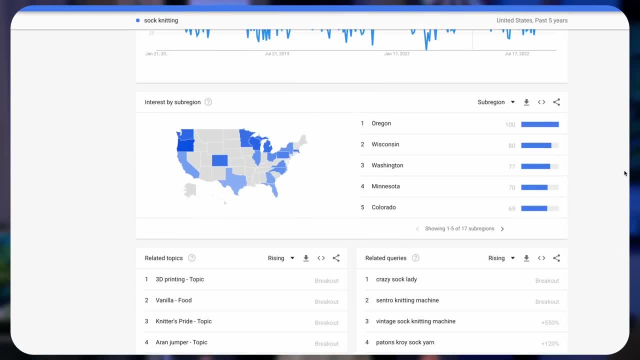 according to Google Trends, it looks like a pretty stable topic over the past 12 months, with a pretty obvious spike in November, Which makes sense, as these are probably a pretty popular gift around the holiday time. So let's take a look at Google Trends. 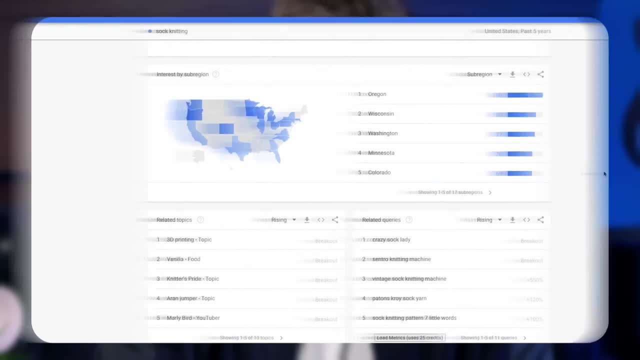 But we can also take a look at it over different timeframes, not to mention breaking it down by different countries and different states. You can also see any related topics or, my personal favorite- related queries, which, in this case, is going to show us the terms. 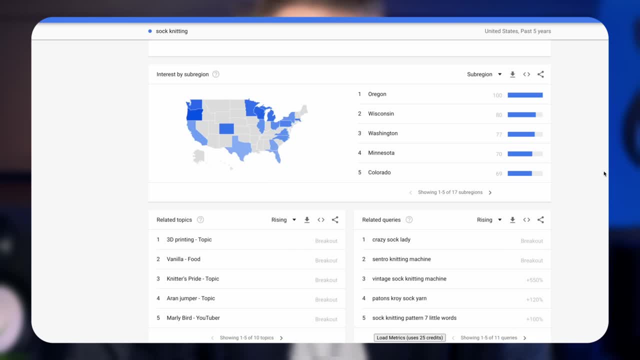 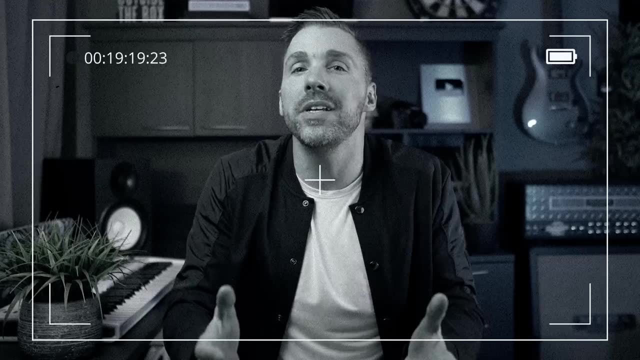 Crazy Sock Lady and Centro Knitting Machine, which are topping the charts with the term Vintage Sock Knitting Machine, showing an increase in interest of 550%. Powerful stuff, and I'm sure I don't need to tell you just how incredibly useful it is to know. 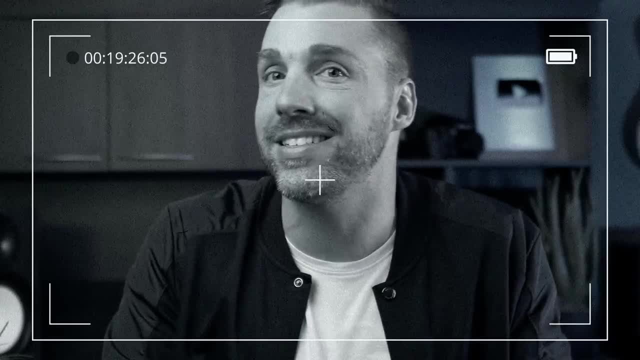 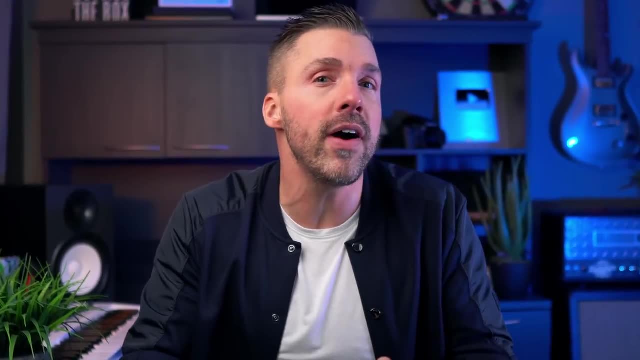 exactly what people are searching for, what they're interested in and the exact keywords that they're using in order to find it Okay. next, let's do a little competitor research in order to dive a little deeper into your competitors and find out if they're really as smart as they think they are. 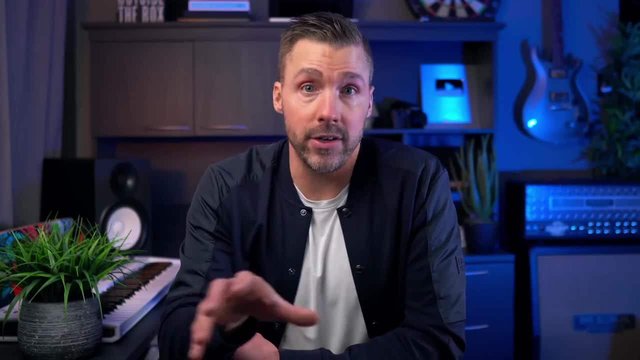 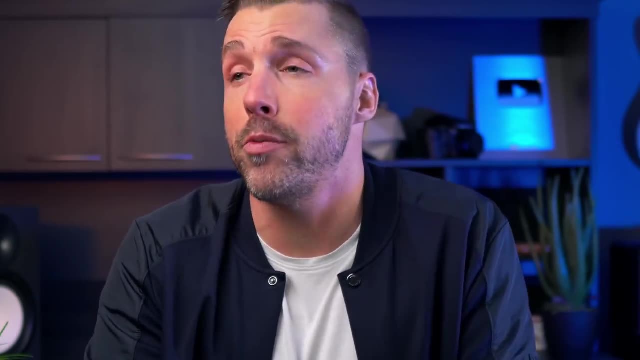 Now there are two big dangers that you need to look out for when you're doing competitor research. The first is not knowing who your competitors are, or ignoring them completely, which is inexcusable and, for lack of a better term, just silly, After all, even if they're doing most things. 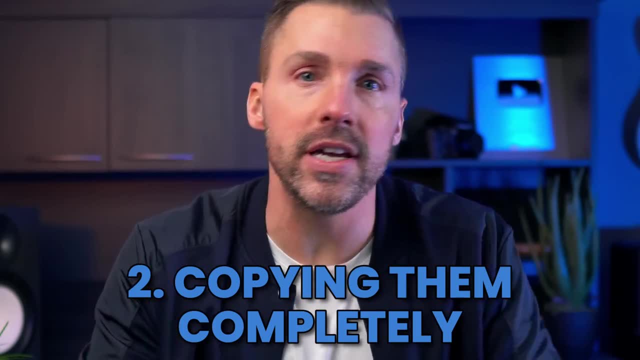 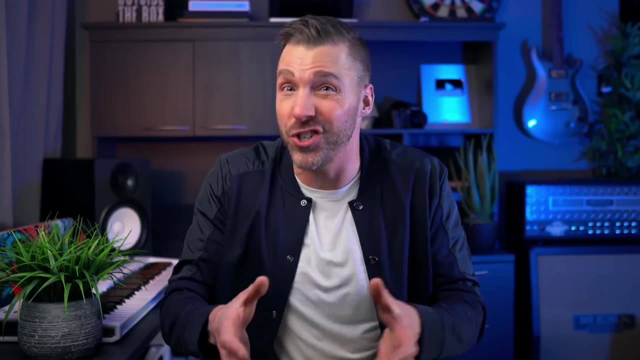 wrong. well, there's still lessons to be learned, And the second danger is copying them completely, which leads you coming off as a second-rate version of them and 99 times out of 100, people are just going to want to go for the original version. 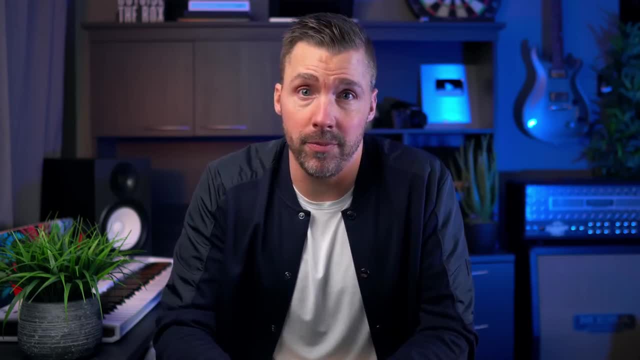 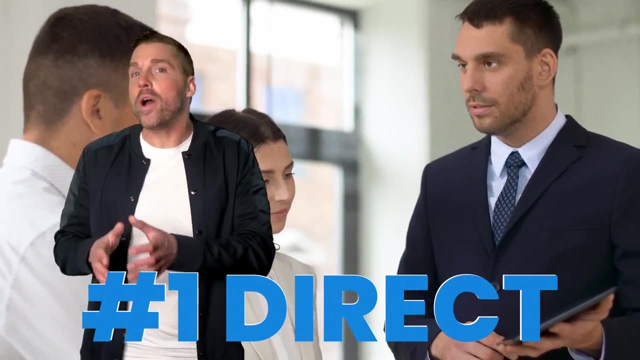 So, with that said, here's how you do competitor research the right way. First off, you need to make a list of your competitors and group them into one of four different groups. Number one is direct. These are people that sell what you sell to who you sell. 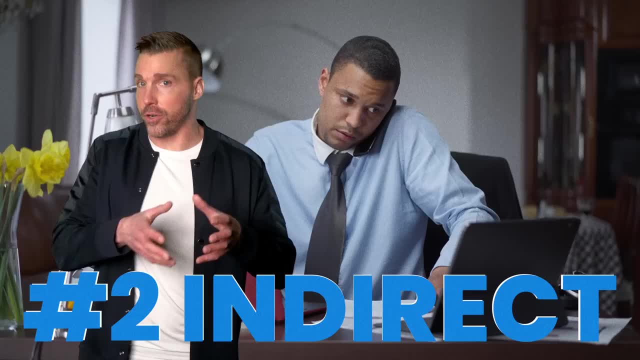 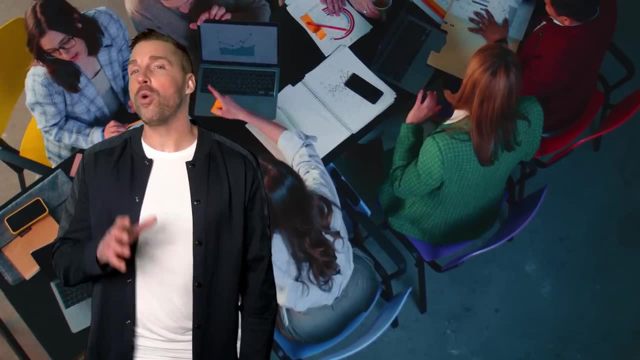 Next is indirect. These are people that sell what you sell to a different group or different segment of the market. Number three is colleagues. These are people that sell something different to who you sell. And number four is futures. These are people that sell something to people who will eventually become your target audience. For example, if you 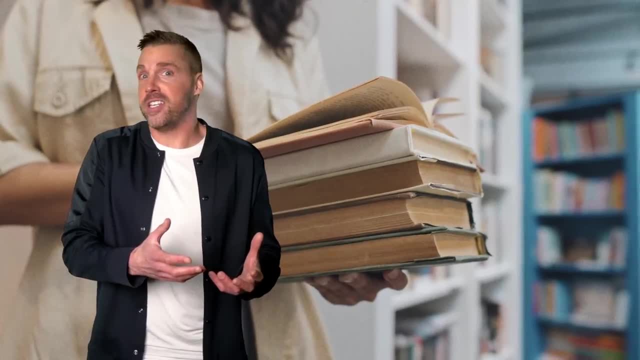 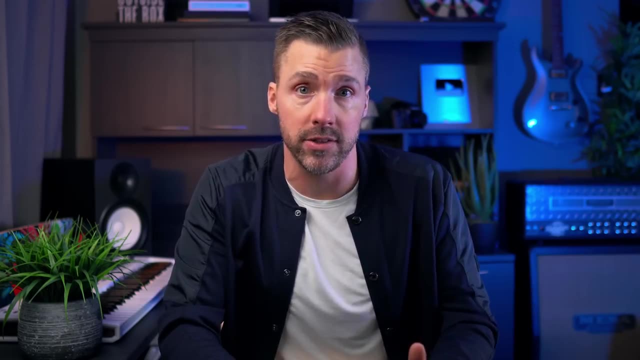 sell running shoes. they may sell walking shoes or books that teach people how to run. Once you have these lists, you want to start diving into their content and their website and their social media profiles. What do they offer, What do they talk about And how do they? 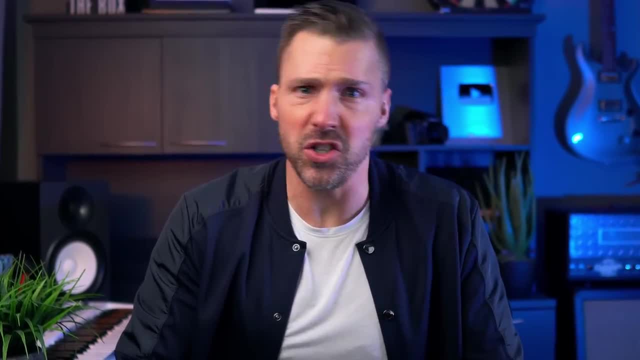 talk about it. Are they cheap, Expensive, Fast, Slow, Boring, Strange, Interesting New Novel, Shiny Tasty. You need to know what's out there so you can know what they're doing and how you're. 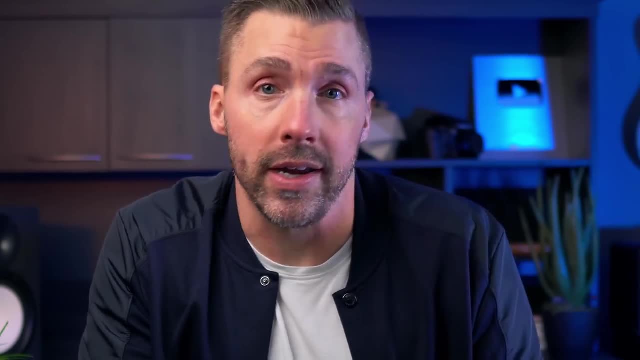 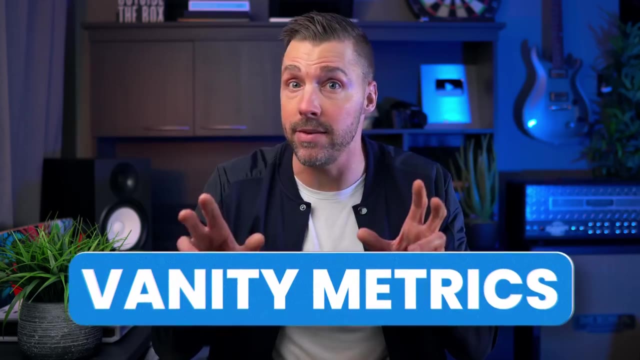 going to differentiate yourself from them, but also so you can see what's working and what's not. So here's the deal on that. While I never advise judging the success of your business or your marketing campaign on vanity metrics such as likes and comments and shares, they do provide. 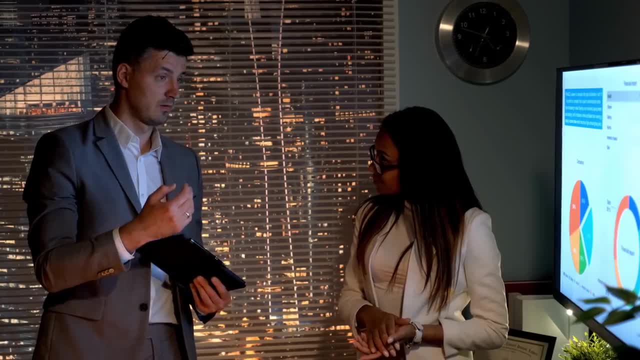 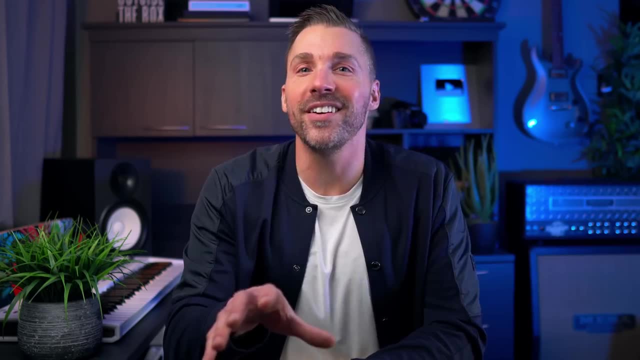 at least a small level of value, at least insofar as figuring out what their audience likes and enjoys, what content they want to see more of and less of. That said, an important point here is there is a very big difference between buyers and non-buyers, And you want to make very sure that. 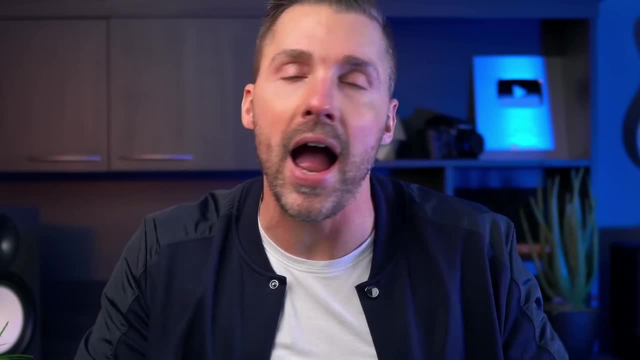 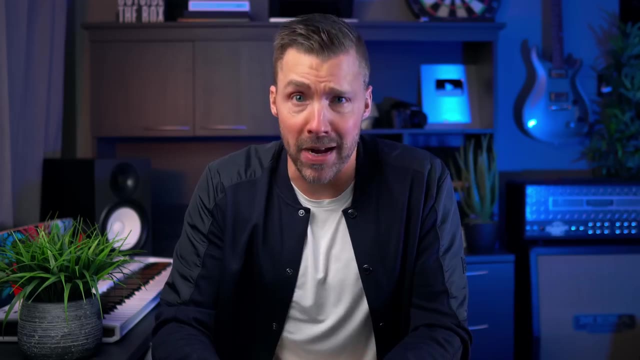 you're basing your business and marketing decisions off of people that are actually willing to pay and buy whatever it is that you're selling, Not just with likes and loves and hugs and high fives, but with money, because that's how business works. So let's talk about that next. 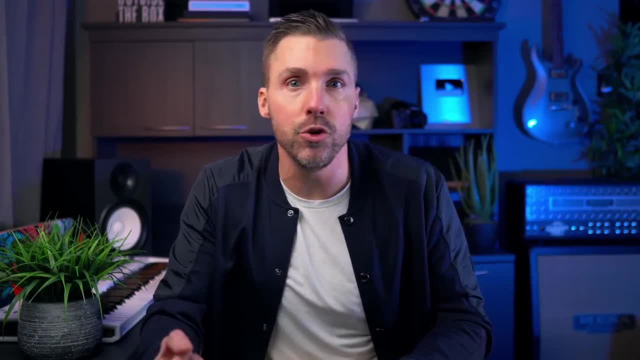 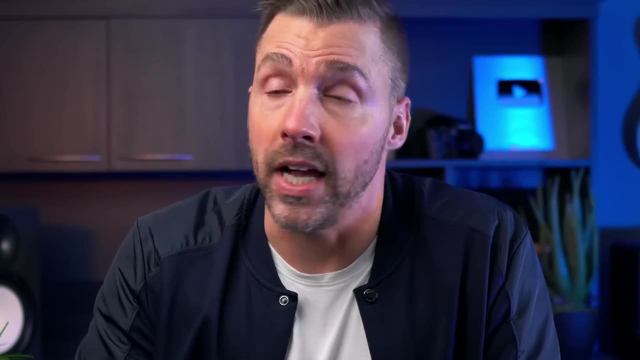 Now full disclosure. if you're in the early stages of launching a new business or starting a new company, then this next part isn't going to apply to you yet, But- and this is a big but, I cannot lie- it's still something that you want to pay attention to Because, moving forward, 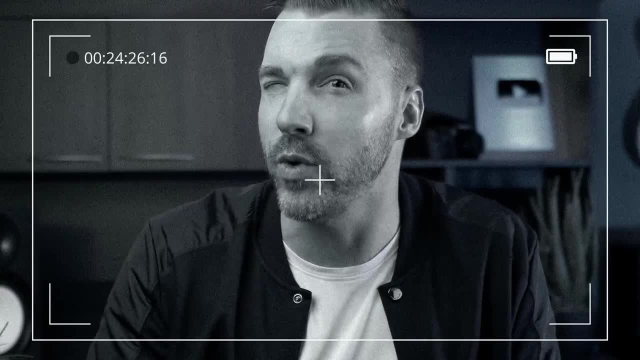 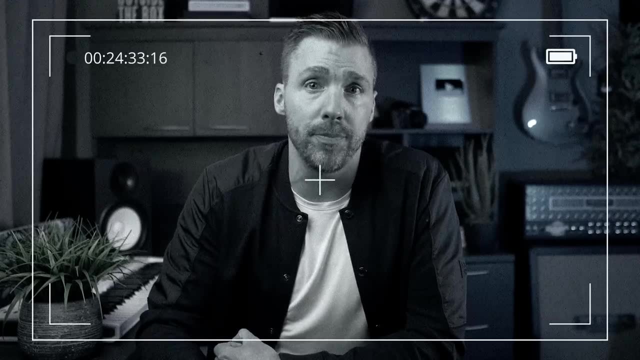 you're going to want to know what to pay attention to and what to be able to ignore in order to give your business, or your startup or new company, or whatever it is that you're launching, the highest likelihood of success possible, And if you happen to already have a business, with current or previous 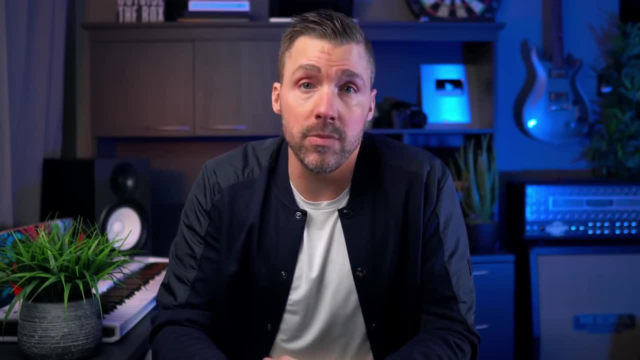 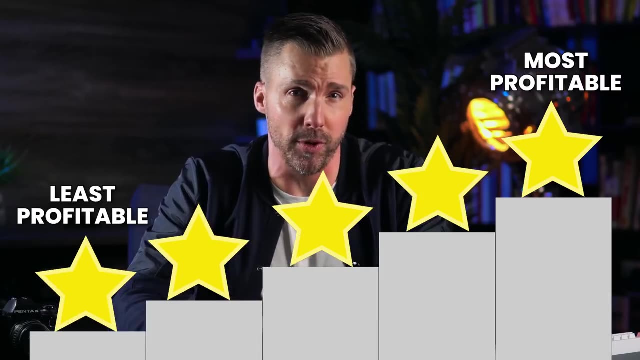 customers, then you, my friend, are sitting on a goldmine, So here's how to make the most of it. First look through your previous and existing customer database and rank your customers from most profitable to least profitable. Then take a look at the list of the most profitable customers. 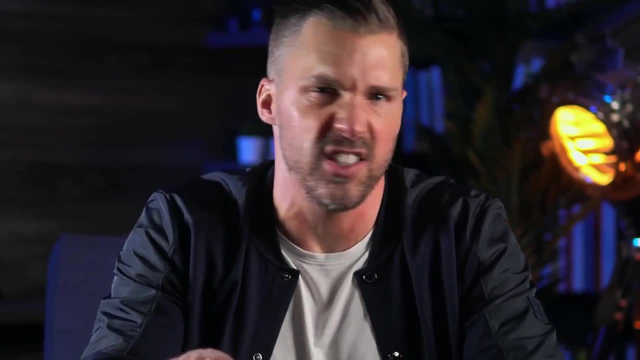 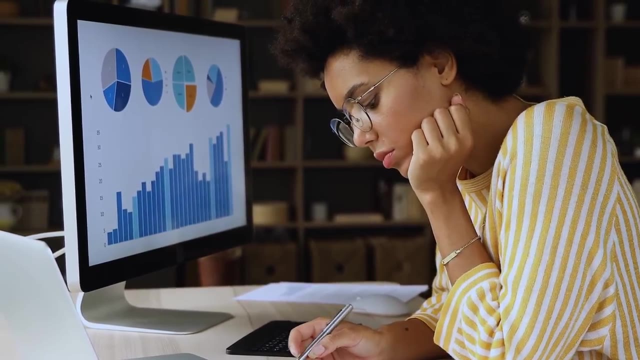 in the world. Take a look at the top 20% of your customers and look for any common trends or themes or characteristics. For example, are they all women or all men? Are they all between the ages of 20 and 30, or 40 and 50?? Do they all buy the same thing And if so, what is it Then? once you have this, 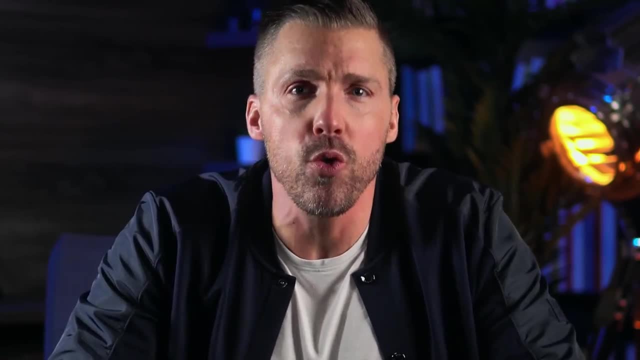 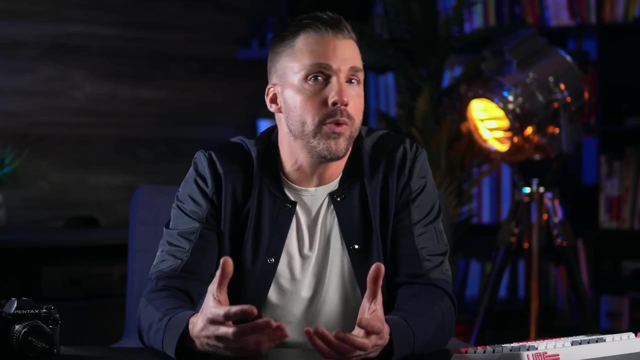 information. dig deeper by seeing if you can talk to them and ask them a few questions about their needs and why they chose you and what they love most about your business. After all, they are your best customers, so it only makes sense to use the answers they give you to build more specific. 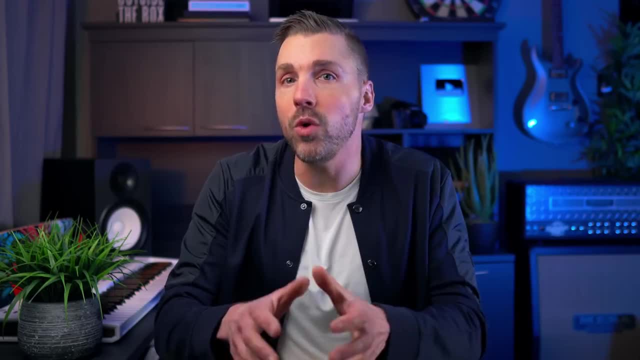 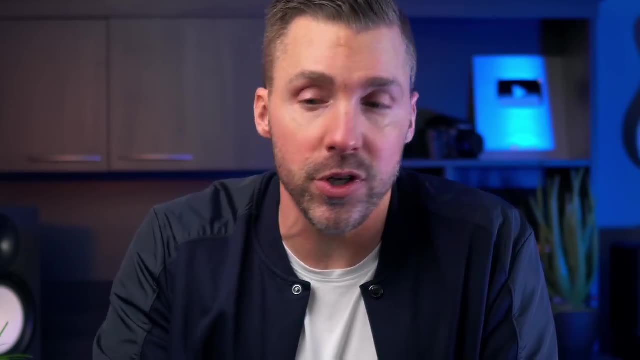 marketing content and messages around them, Of course, if you don't have the option to talk to them or you don't have any customers at all. yet there's still another incredibly powerful market research tool that you can use right now in order to get nearly instant feedback.